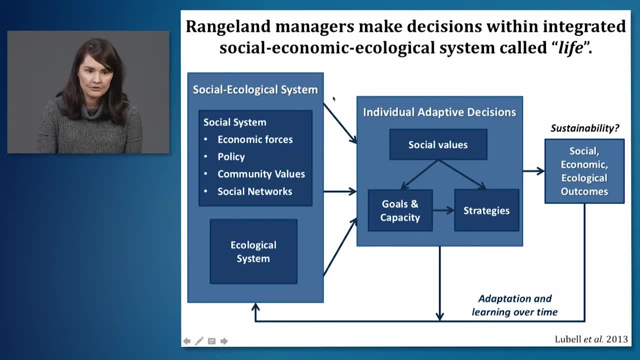 and social networks, for example, which all interact to shape and affect the individual adaptive decisions, the social values, goals and capacities and strategies of individual operations, which in turn influence the social, economic and ecological outcomes. And over time, we have feedbacks, adaptation and learning. 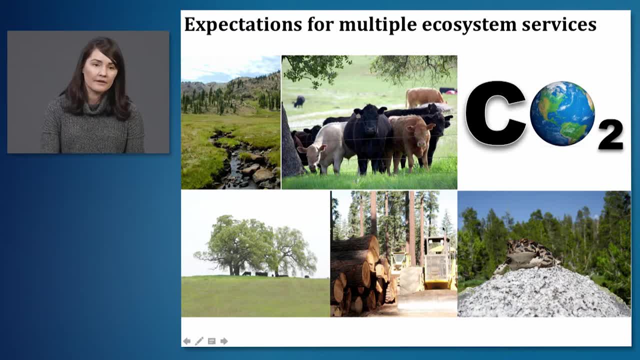 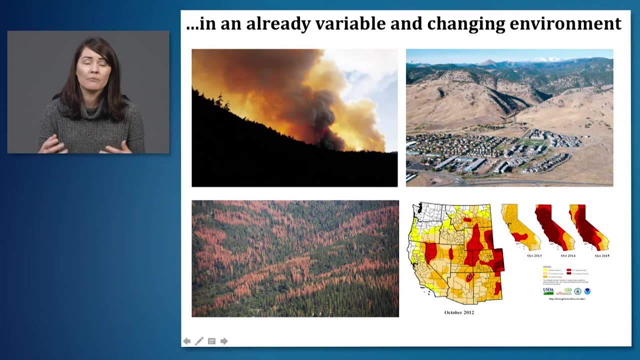 On top of all of this complexity, of all the biophysical and social complexity, we also want more, And we're seeing expanding expectations for multiple ecosystem services from these rangeland landscapes. On top of that, we're already wanting more in an already variable. 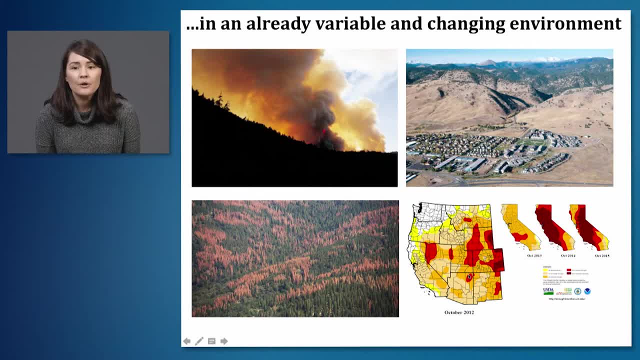 and changing environment, and this is particularly challenging with the mounting pressures of global environmental change, including altered fire regimes, development in the urban-wildland interface, the spread of disease and invasive species, and prolonged and severe droughts- And California is on the leading edge of many things and drought. 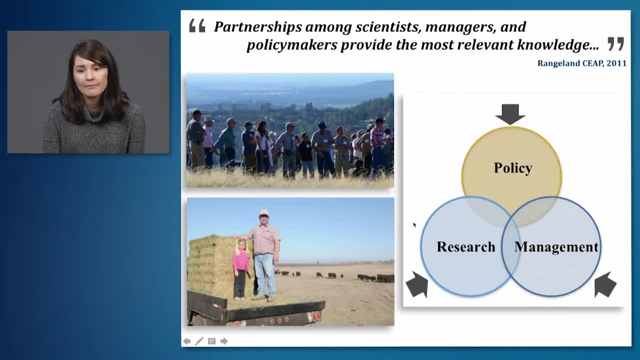 is no exception. So if we're going to think about how we want to adapt to a changing environment and cope with these challenges, then we need to understand the social context, the place-based perspectives and experiences of those who live and work on these lands, And so that we can better bring together the 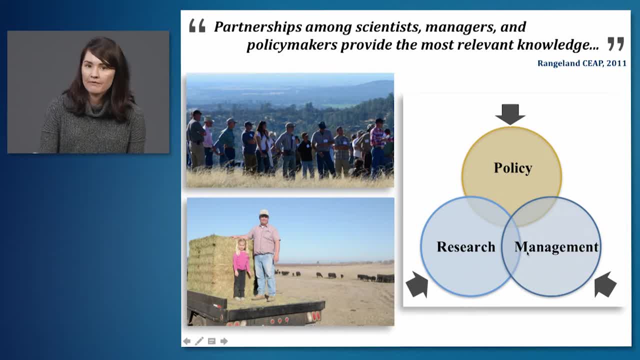 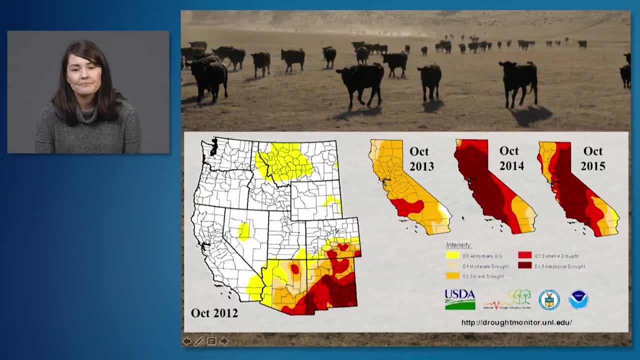 policy, research and management realms to better provide the most relevant knowledge, And a good place to start to do this is with the experienced resource managers themselves. Unlike other natural hazards, drought is a gradual, complex disaster with very indistinct starting and ending points. Severe and widespread. 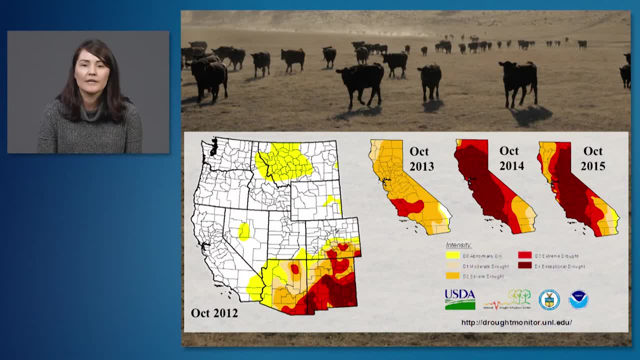 droughts can trigger massive undesirable ecological shifts, which can impact forage and livestock production capacity and directly threaten livelihoods. The communities reliant on rain-fed rangelands are potentially the most vulnerable to climate variability, given their dependence on such a climate sensitive resource, And, in fact, rangeland livestock producers are among. 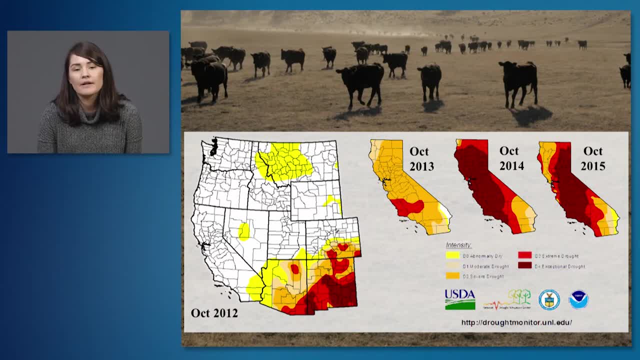 the first in the agricultural community that is often affected by drought. Drought has played a formative role in California's early history and has continued to do so with at least six multi-year droughts since 1960, including our very recent historic statewide drought. 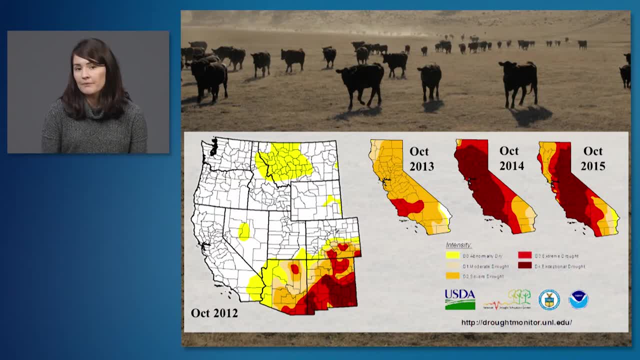 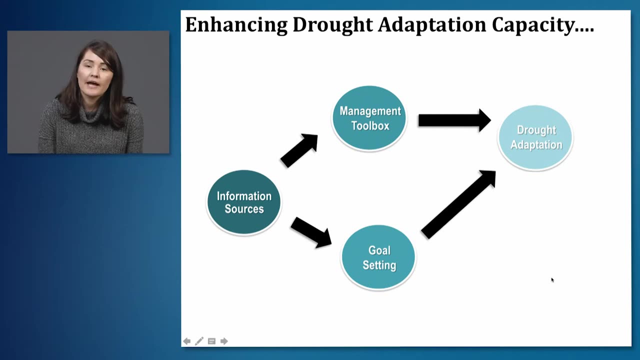 So, with most family operations in California- family ranching operations being three generations or more in ranching, there's a lot of experience here that we can learn from, And we can particularly learn how we can effectively enhance drought adaptation capacity which, as we know from our 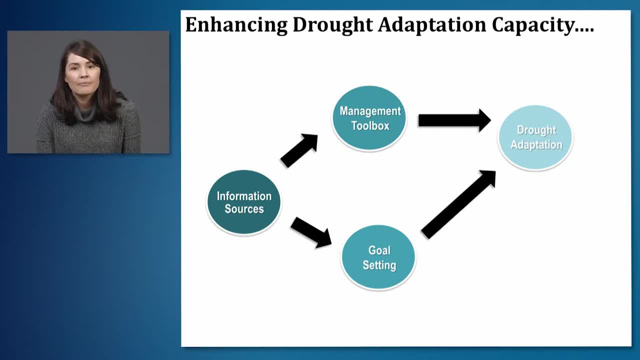 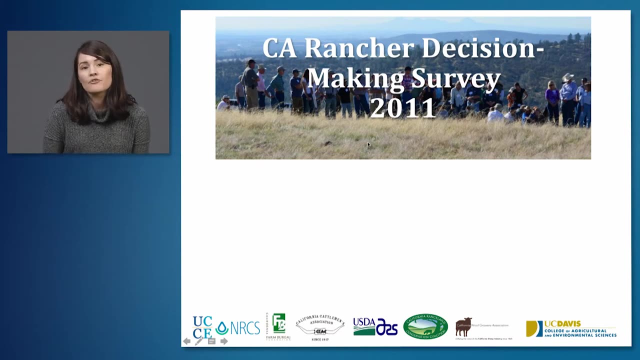 adaptive decision-making work can potentially be influenced by a host of decision-making factors, including information resources, goal setting and management capacity, or the management capacity, So we can learn from those and we can make a difference in the management toolbox. To this end, we launched a series of survey efforts, working with the 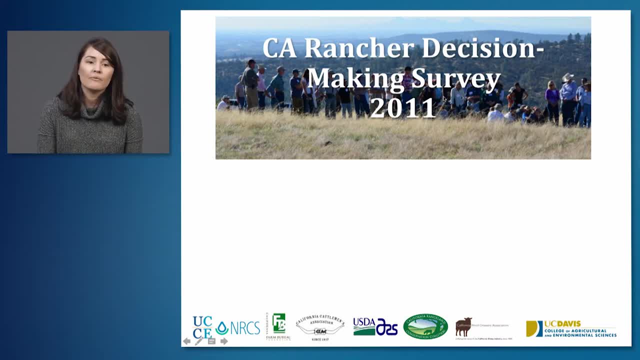 California ranching community, starting with the California Rancher Decision Making Mail Survey of 500 ranchers across the state, And this survey focused on several themes including operator and operation demographics, information, resources and operator values and beliefs, management goals and practices. 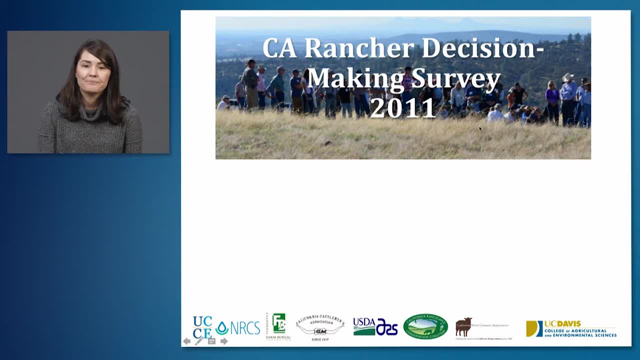 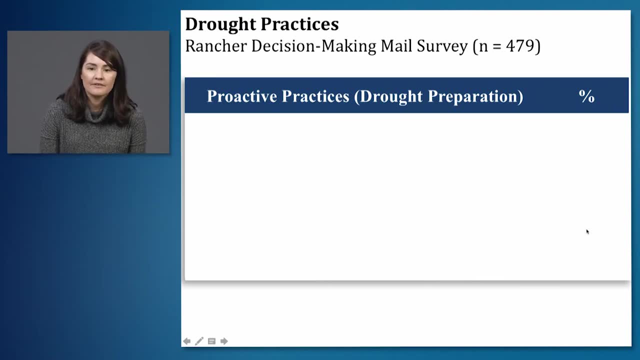 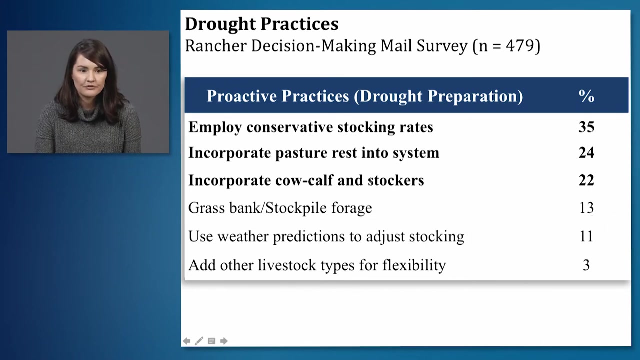 and specifically focused on management for drought. In terms of drought management practices, we specifically asked about proactive practices. proactive drought management practices- What are the practices that managers used to plan for potential drought in the future? And what we found was that the primary tools, or the top three tools here in bold, really focused. 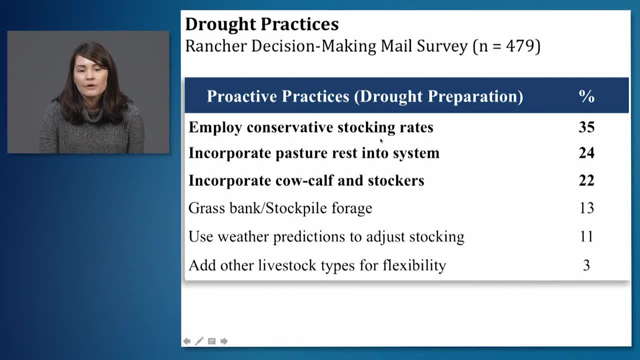 on conserving forage and actively managing risk. So the top practice was employing conservative stock And we found that the top three tools were stocking rates, which 35% of ranchers do- In terms of setting the stocking rates based on expected forage supply during less favorable years or dry or drought years, so that they can reduce. 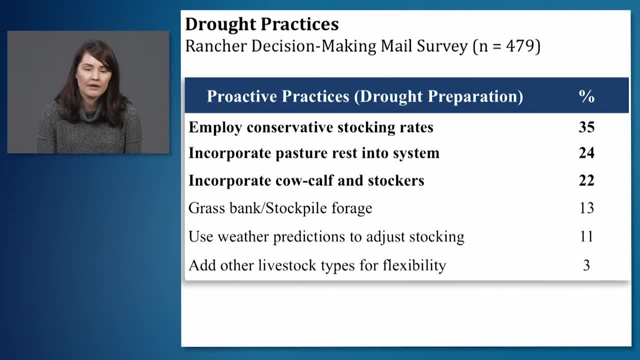 the chances of having to sell animals during periods of unfavorable price markets. The second most popular was pasture rest. incorporating pasture rest into the system- About 24% of ranchers said they do this, and allowing pastures to rest allows them to recover and save and provide. 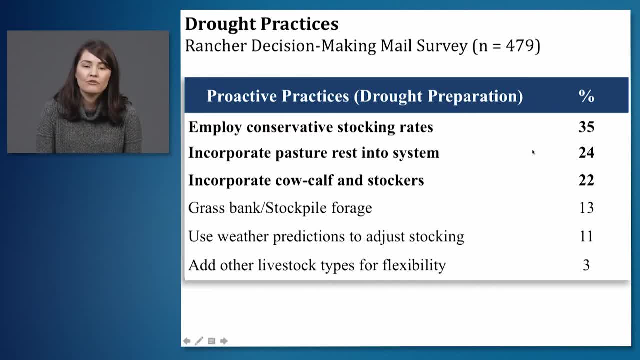 future forage resources. Also, about 22% of ranchers add what we can think of as a relief valve to the operation in which they integrate multiple classes of animals- here cow-calf, as well as younger yearling stocker animals, which allows them to be more flexible in their overall herd. numbers. We also have a lot of ranchers that do this, and we have a lot of ranchers that do this and we. We also have a lot of ranchers that do this, and we have a lot of ranchers that do this, and we. 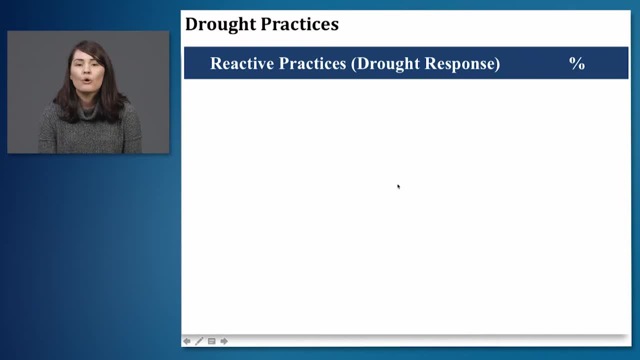 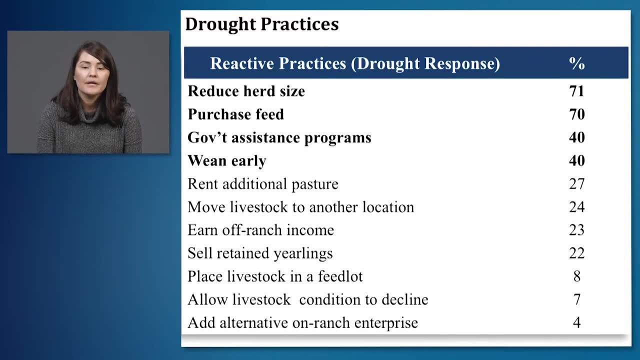 also asked about reactive drought management practices. So what are the practices that ranchers use to respond to a current and ongoing drought? In terms of the primary tools or the most utilized practices across California, they tended to focus on managing impact to the bottom line. 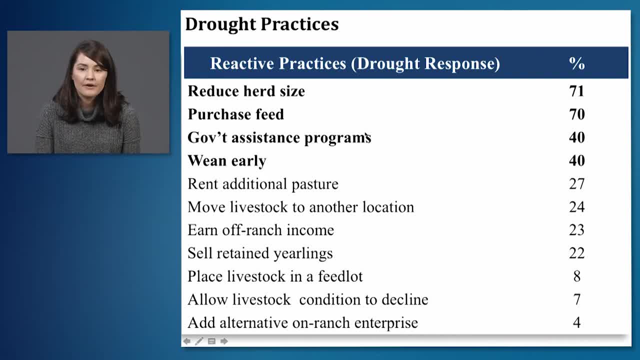 not surprisingly, Over 70% of ranchers said that they automatically immediately reduced the herd size or per capita. So we have a lot of ranchers that do this and we have a lot of ranchers that, in turn, encourage ranchers to purchase feed to maintain their core herd. 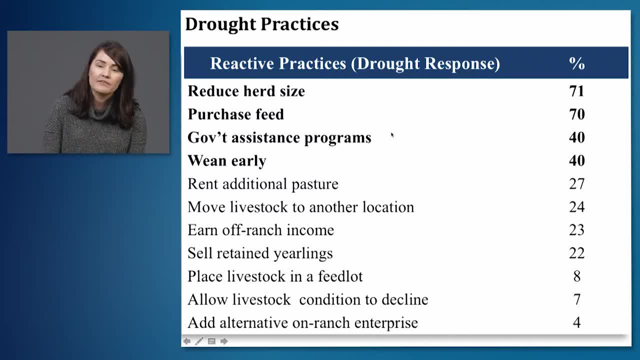 The third most utilized practice was the use of government assistance programs such as disaster relief, with 40% of ranchers and another 40% of ranchers said that they use early weaning to reduce demands on mother cows when they're in their critical energy and nutrient requirement periods. 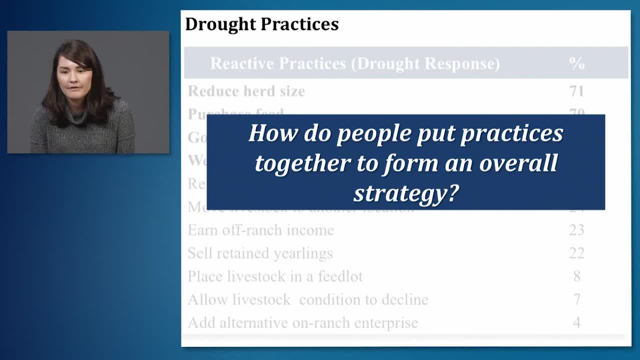 And so those are the most commonly used reactive and proactive practices that we found in foodfarms. So those are the most commonly used reactive and proactive practices that we found, as foodfarms and products have been working differently across the差s. So as we turn into health care, there are a number of 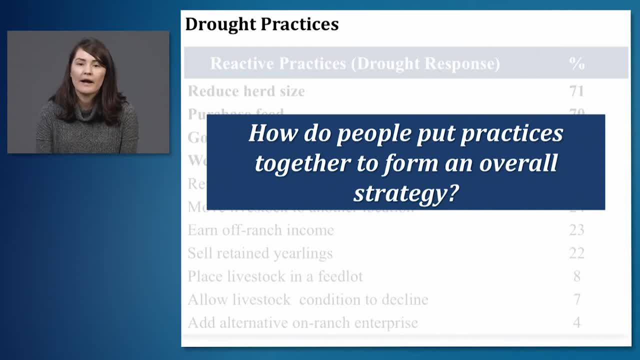 sort of think of them as the seven primary or core practices identified. But we also wanted to know: do ranchers- a lot of them- use a lot of the same practices, but do they put them together in the same ways? Do they use the same suite of practices or is there variability across operations? 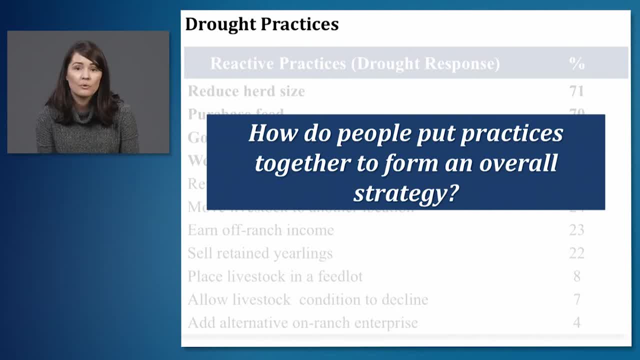 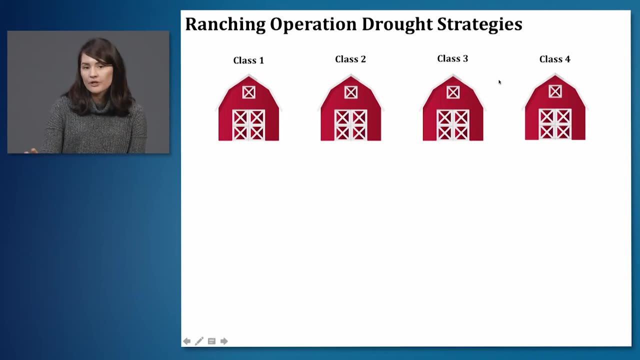 And so, based on rancher responses to those individual practice questions, focusing on reactive and proactive drought practices, we statistically identified classes of drought strategies that people use across California, And when we did this we found that generally there are four broad classes or types of on-ranch drought management strategies that operations can be classified into. 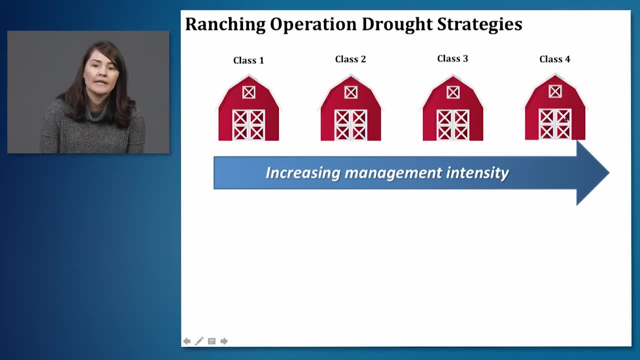 And these resulting classes span a gradient of increasing management intensity, or you can think of it as correlated to number of practices used, with class one being the least intensive management practices used and class four having the greatest management intensity. And to give you an idea of some of the identifying practices, 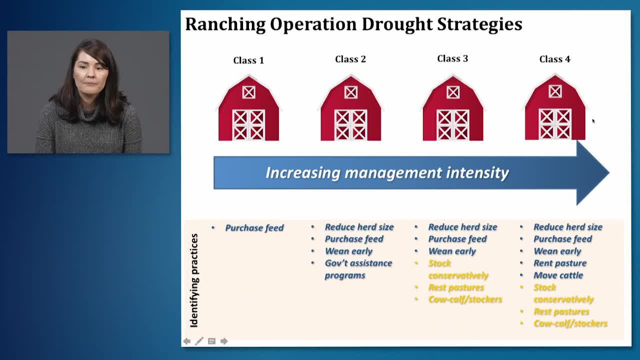 and characteristics of these types of classes. we found that classes ordered ranged from class one here, which had very low adoption rates of any drought management practices. In fact, these tended to be smaller operations with no prior experience with drought. This ranged from class one. as we move along this gradient to classes, 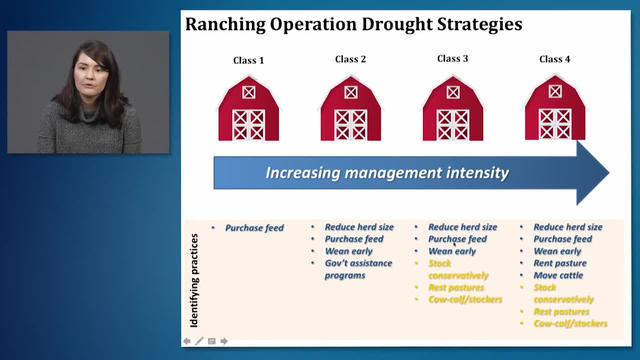 with larger numbers of drought management practices used and increasing emphasis on proactive practices, which you can see here in yellow as we move along this gradient. And these classes, particularly classes three and four. they tended to be larger operations with access to more resources. 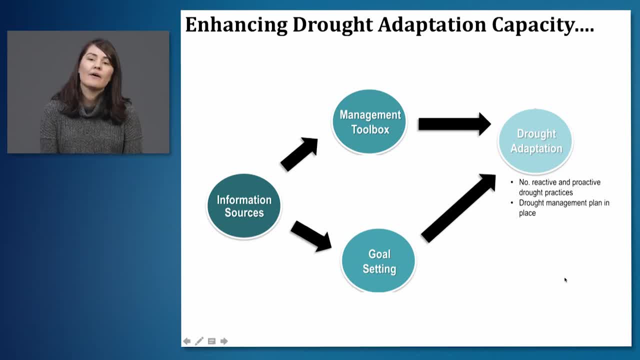 In terms of how we can use these classes, in terms of how individual drought adaptation is enhanced by those decision-making factors. we define drought adaptation capacity by the number of drought practices, both reactive and proactive, because, as we just saw, that's very important in defining the drought management strategies. 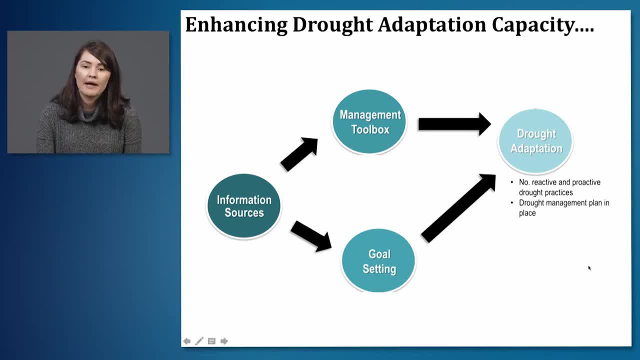 across California, as well as defining it by whether people had a drought management plan in place, whether they were doing active drought planning, And what we found was that, indeed, drought adaptation capacity was enhanced by information resources. so indicators like formal education level, as well as access to high quality and a high number, 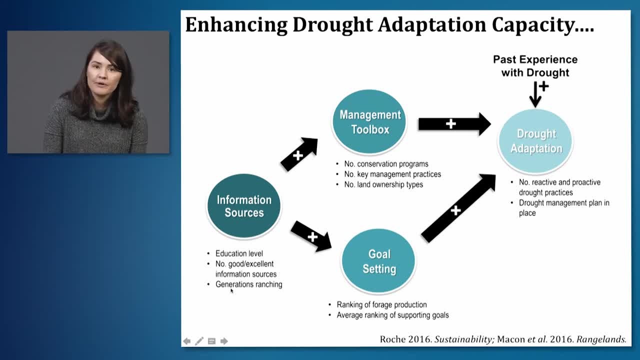 of information resources and a large number of generations in place on the ranch to contribute to that knowledge source. We also found that goal setting also enhanced drought adaptation capacity. So, for example, people valuing the future forage resources and ranking forage production very highly among their ranching goals. 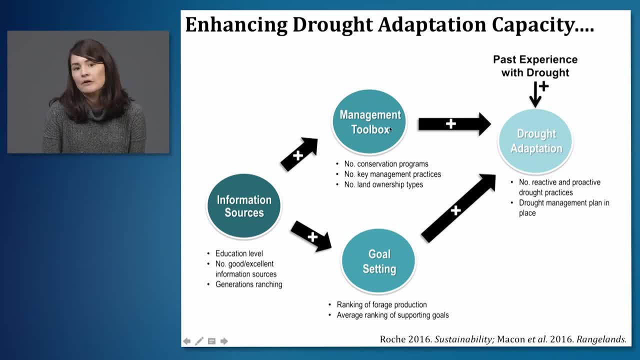 The management toolbox was also very important and positively correlated to drought adaptation capacity. Having the flexibility in those resources, such as having multiple land ownership types, allowed them to be able to adapt and cope with drought more effectively, And we also found- not surprisingly- 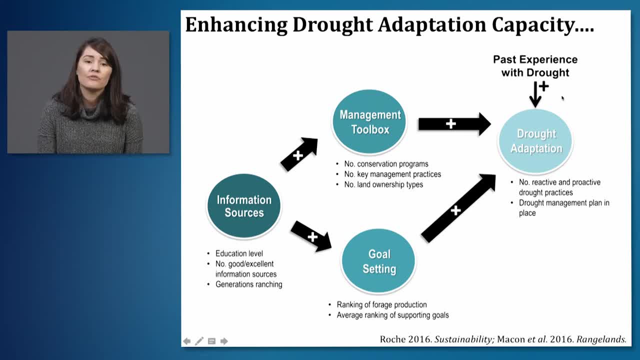 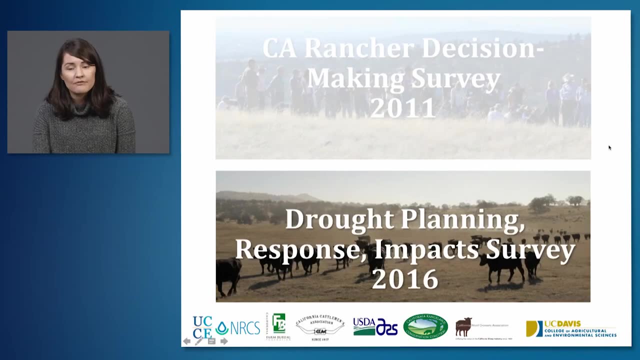 as we saw with the drought management strategies, that past experiences- the past experience with drought- was also positively correlated with drought adaptation capacity. So those that had experienced drought in the past were more able to adapt to and cope with drought. So that's what we learned about ranchers' past experience with drought prior. 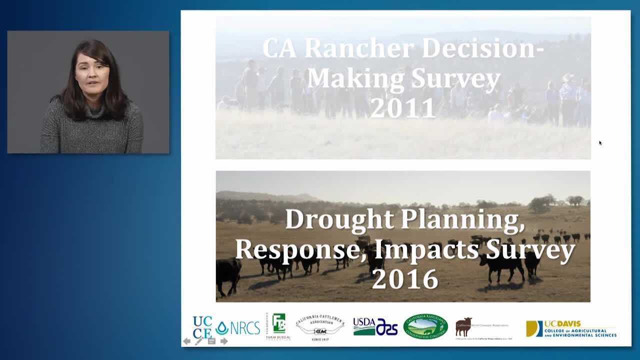 to California's 500-year historic drought. Most recently, we looked at what have been some of the changes in management practices following the onset of that historic drought and we worked with a subset of producers, including cattle and sheep ranchers across California. 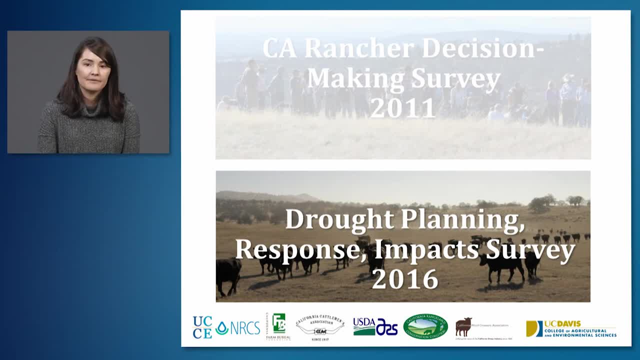 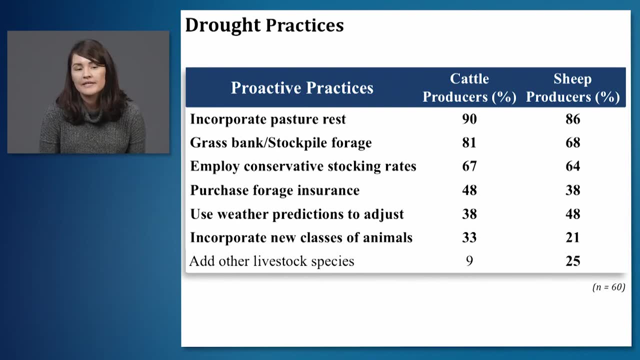 to better understand drought planning responses and impacts In terms of drought practices. we asked many of the similar questions that we did in the 2011 survey and we found- for cattle producers in particular, we found increased use across the board. 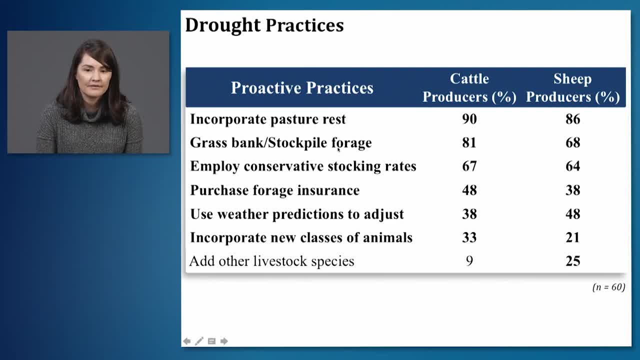 as well as a broader diversity of primary practices for proactive drought management. In fact, we saw as much as 90% of proactive practices used, compared to those much lower rates of adoption prior to the state's historic drought. If you recall the primary proactive practices: adoption. 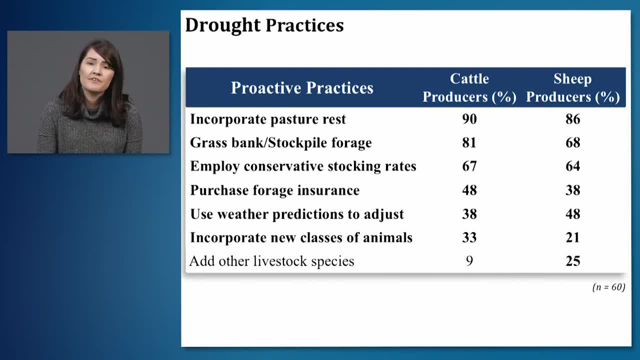 rates hovered around 30%. In terms of differences between cattle producers and sheep producers, we found that cattle producers had greater rates of adoption of grass banking or stockpiling and forage, so saving forage resources for the future, while sheep producers had greater adoption rates. 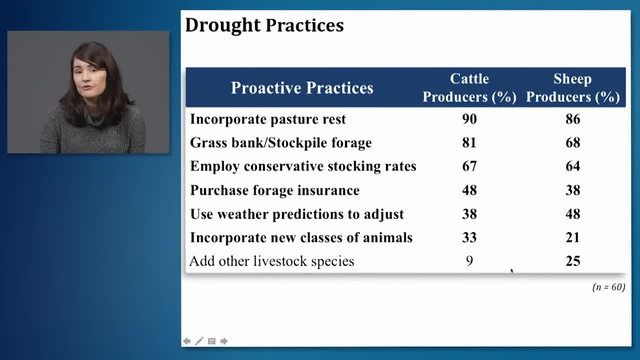 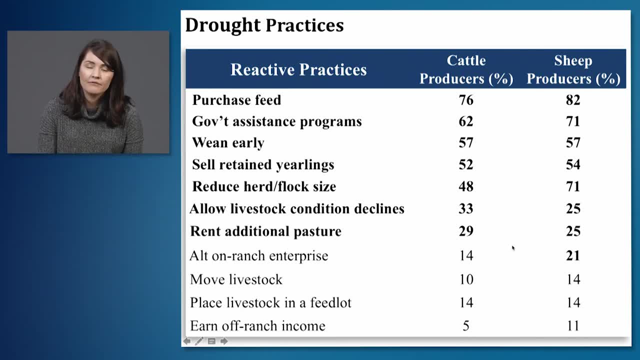 of incorporating other livestock species compared to those cattle producers. For the reactive drought management practices we again for cattle producers we saw increased use across the board with a broader diversity of primary practices here in bold used by those cattle producers In total for reactive and proactive practices. 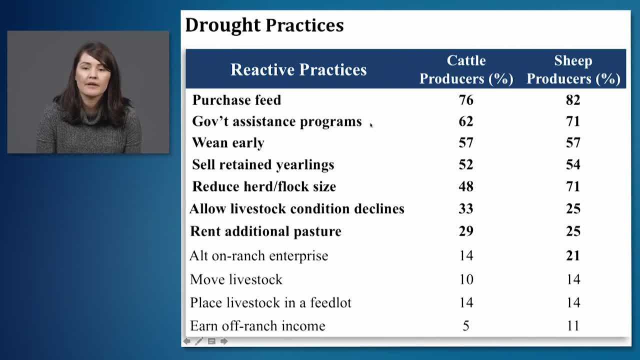 we saw a nearly doubling of the core practices that producers are depending on for drought management after the historic drought. Sheep and cattle producers were generally very similar in terms of their use of reactive drought management practices. with a few exceptions, including sheep producers tended to utilize more the reducing a herd or flock size practice. 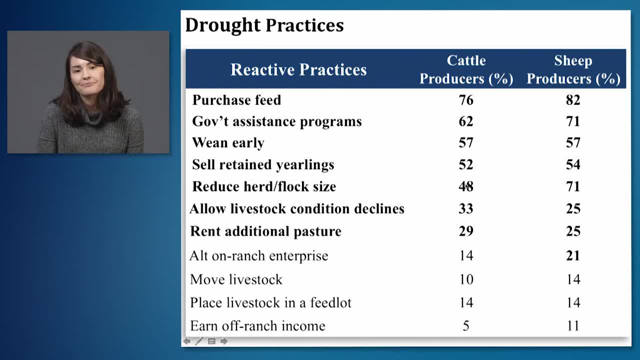 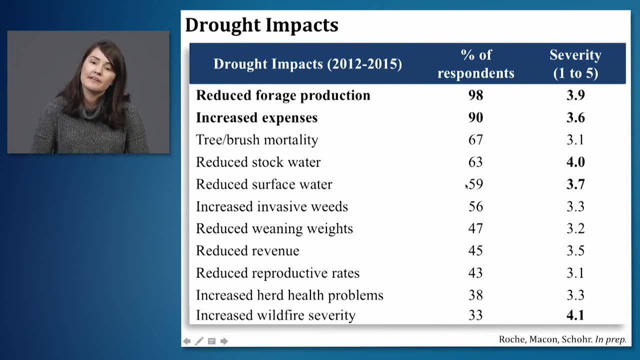 within their operations, compared to cattle producers. In terms of drought impacts, we asked producers what were the impacts that they specifically saw during this historic drought and then what were the severity of those impacts. So we asked them to rank the severity on a scale of 1 to 5,.